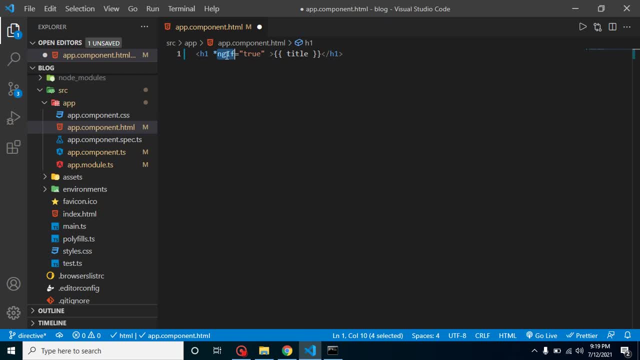 Alright, so how we can define a directive? So see, directives are the classes that can provide some additional feature to our HTML elements. So what kind of additional element? They can overwrite the style, They can just change the text Or some other things, like they can just display our HTML element multiple times, like ng4.. 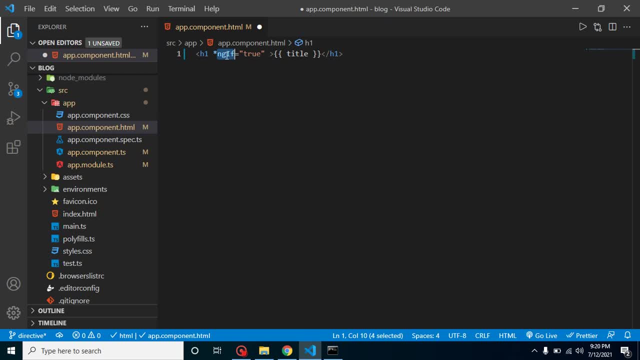 They can toggle our elements, They can hide and show our elements. So these kind of properties or you can see that the additional features can provided by the directives to our HTML element. Alright, so now, how we can create a new HTML, how we can create a new Angular directive. 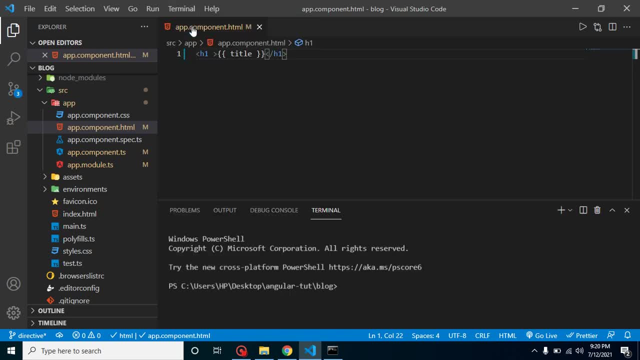 So for that we need to open our terminal And just simply write here: ng g4- generate note nh. ng g4- generate directive and our directive name. So I am just going to put a directive. name is red element. 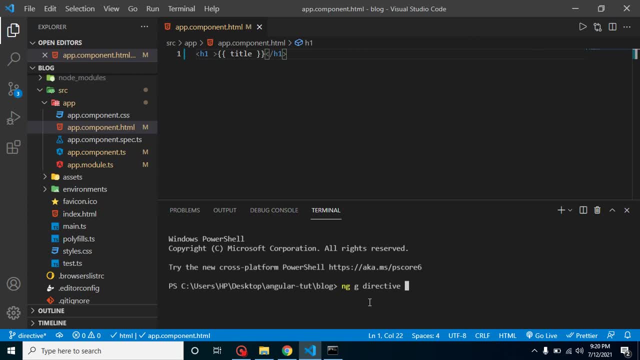 Because, with the help of directive, I will change the style of our element So you can see that red e l And let's enter. So after that you will find that two new elements, New files, are created. 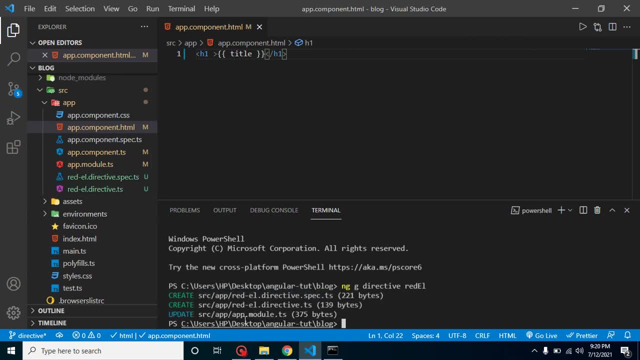 One for directive, second one for testing file of directive, And it will automatically include in our appmodulets also. So we don't need this command line for a moment. So I can just close this panel And now how we can use it. 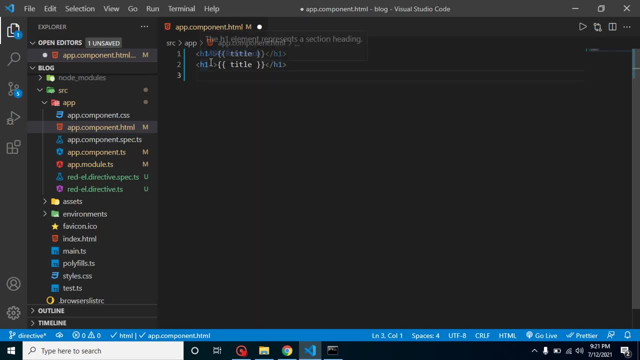 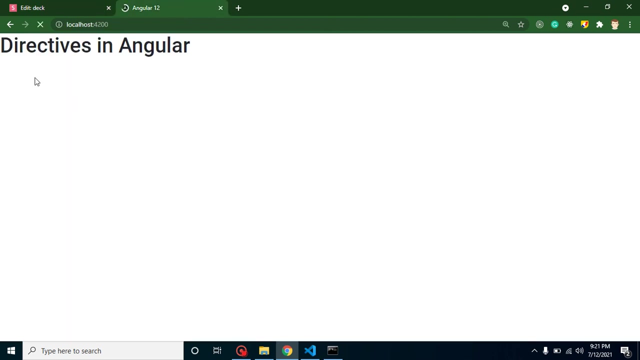 Before that, I want to show its impact, How it can change. So I will just change this. put this red element directive here And it will change the property of our HTML element. So for a, by default, You will find that the both html1 tag have the similar output. 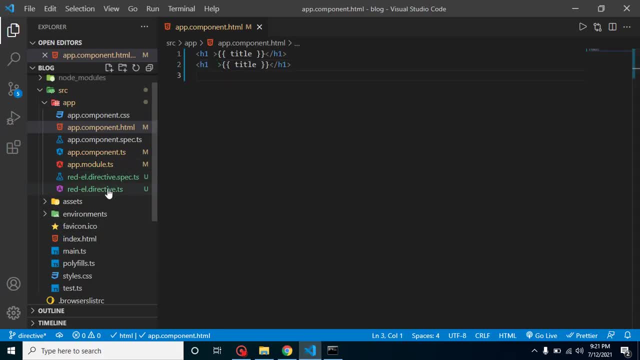 These are the very basic, So how we can apply the directive. First question is that: So here we have a selector, So just copy this selector and just simply apply it here. All right, After applying you will find that that's okay.